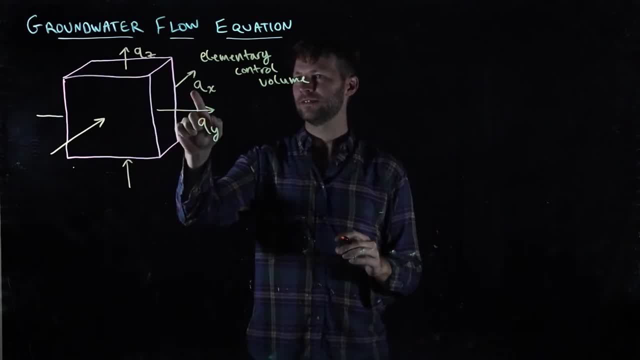 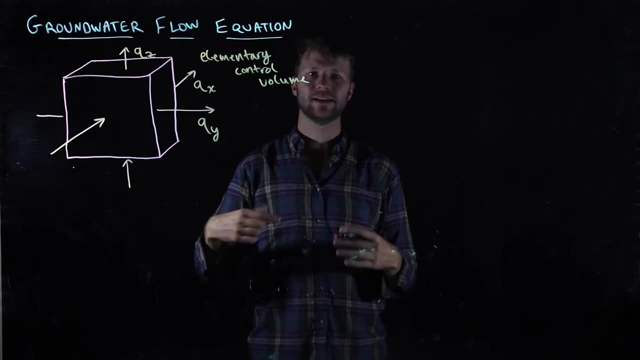 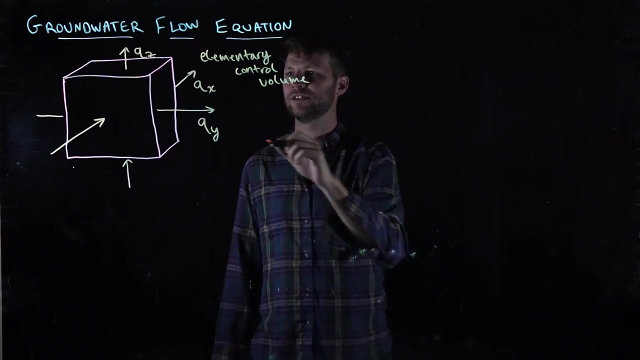 is going to be related to the flow, is going to be related to the difference between the Qx coming in and the Qx going out, So the out minus the in here. And we can describe that mathematically using partial derivatives and describing the change in space here. 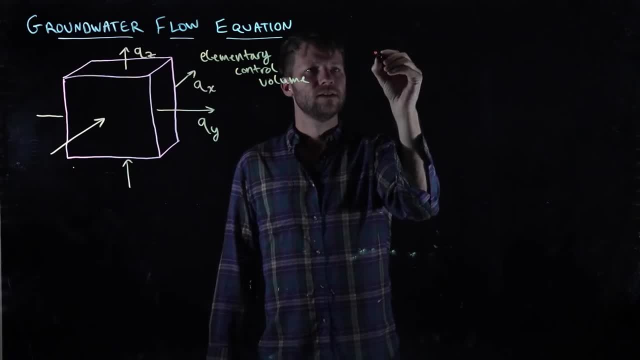 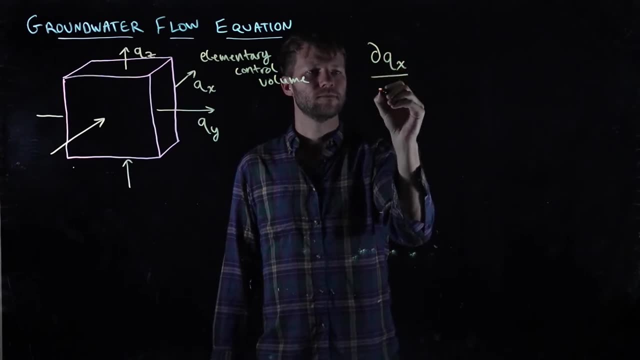 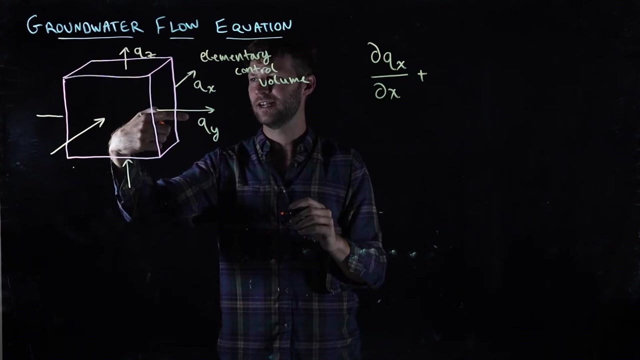 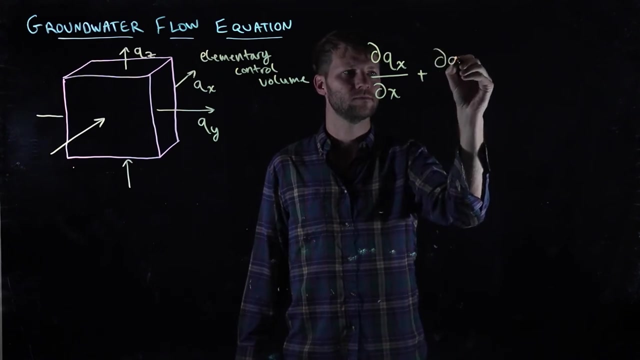 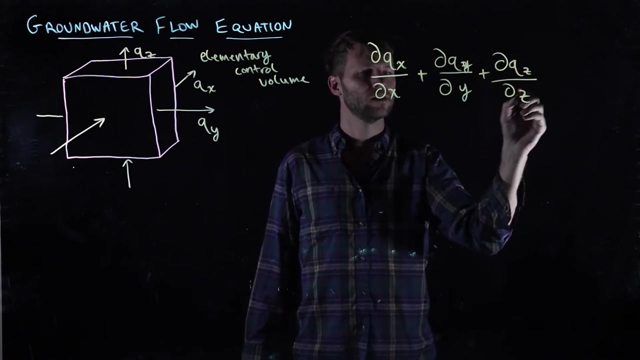 So let's see here- And we're going to add it up in each direction, So we're going to consider the spatial gradient and flow in the x, the y and the z direction. We got a y. So this is describing the output minus the input. 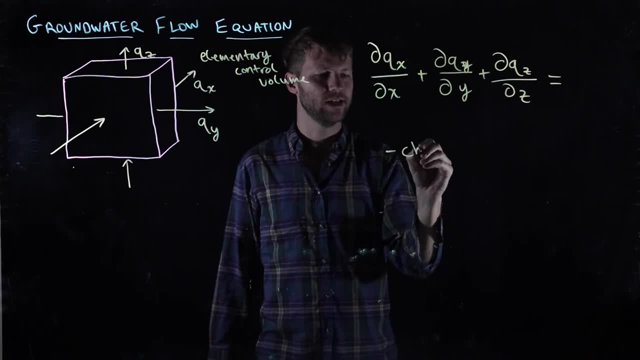 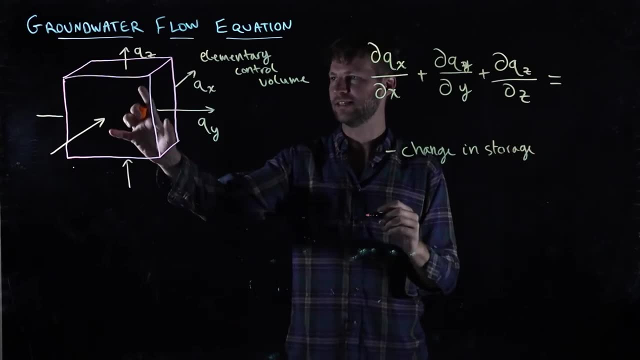 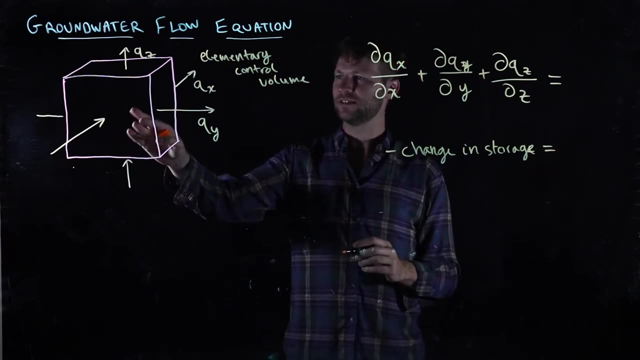 This has to equal the change in storage or the change in mass, if we were to look at the density and the volume here, And we can relate this to the properties of the aquifer. If there's an increase or decrease in storage here, it must mean that water was added to or released from this control volume. 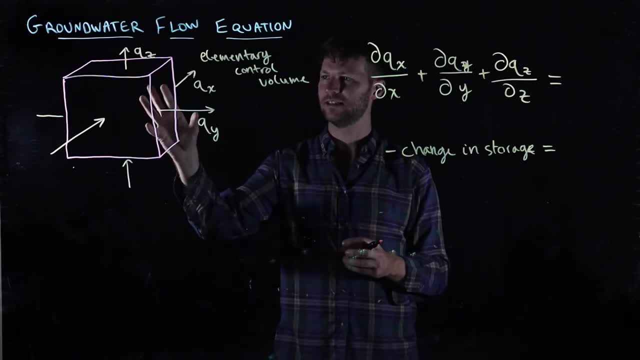 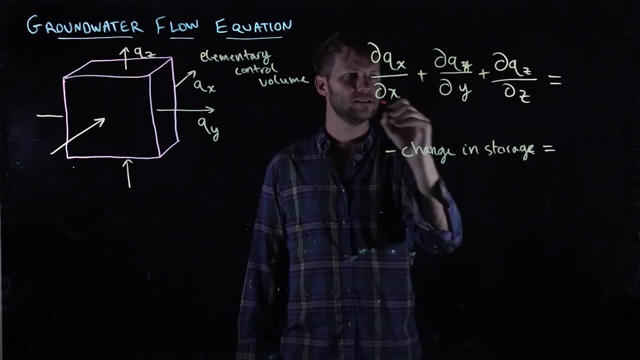 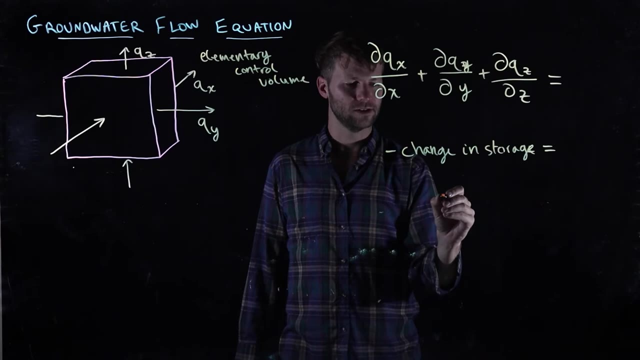 And that has to be related to a change in the head of the aquifer. So the relationship is that these fluxes the in and out, their relationship to the change in storage is going to be related to the specific storage which describes the volume of water gained or released. 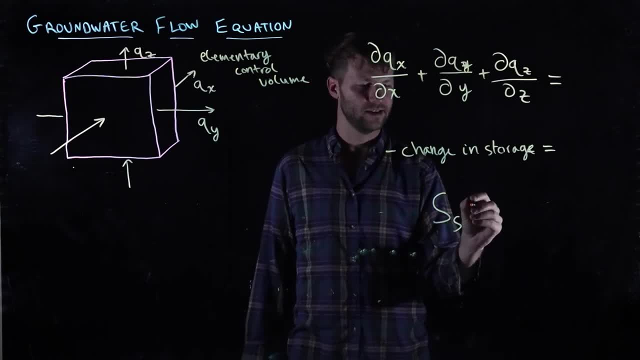 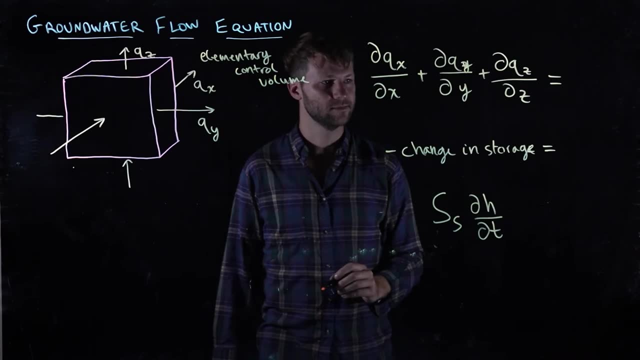 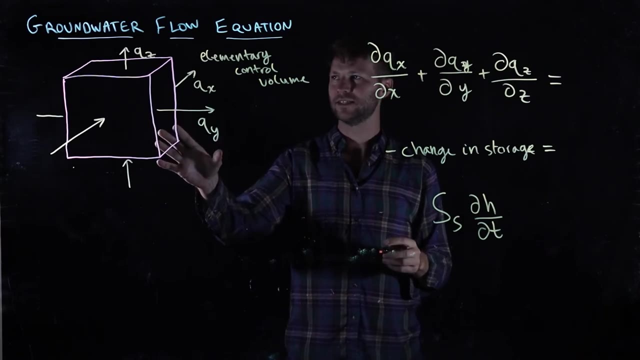 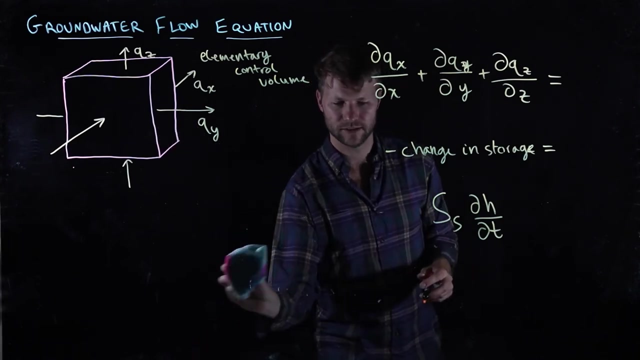 per volume of aquifer, per change in head times, any change in head in time, Just like this. So this is the start of a distribution, A generic form of the groundwater flow equations, given this particular control volume. Now there's one other substitution that we can make here. 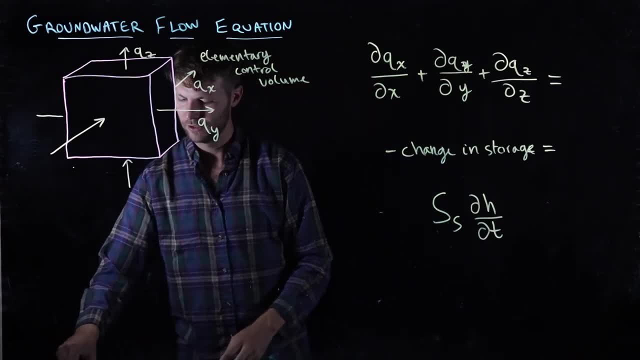 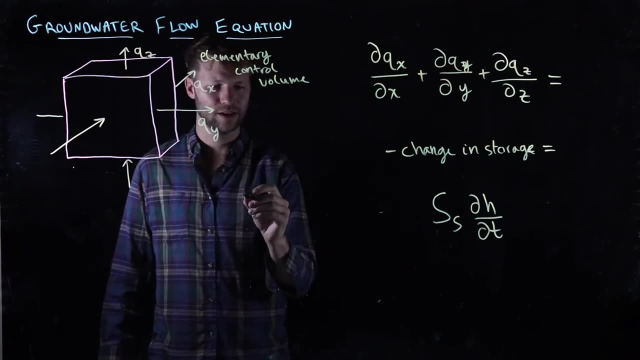 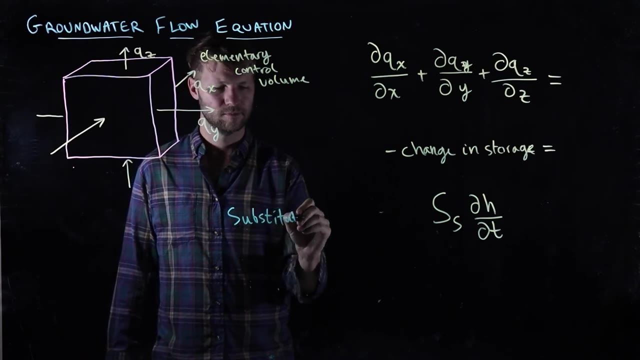 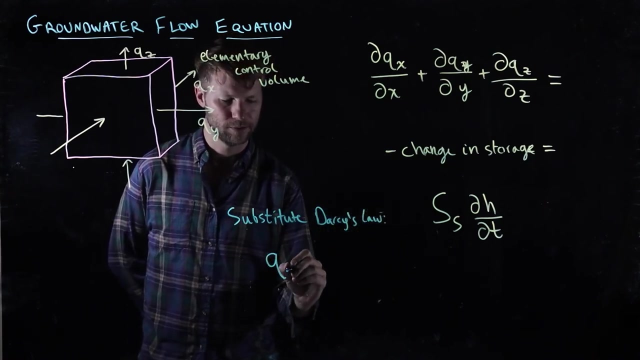 And that is that we know how to express q also in terms of head right. We know, for example, that we could substitute in Darcy's law in this equation And for example, in the x direction, we know that the specific discharge q, sub x.